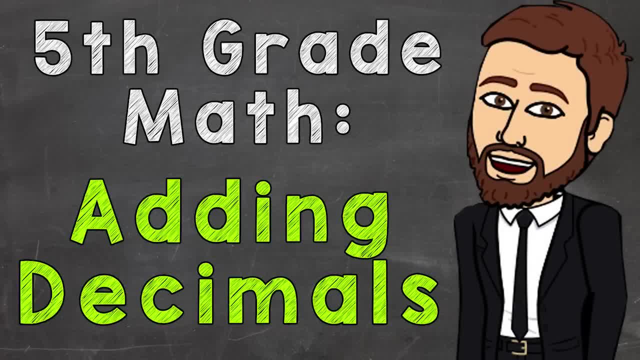 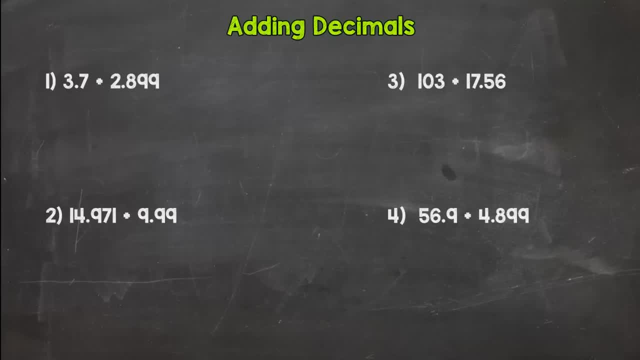 What is going on? Welcome to adding decimals, where, of course, we're gonna be learning how to add decimals. So this is more of an instructional video on how to add decimals, and then we're gonna follow this up with a mastery check where you see if you have it down. Adding decimals is very similar to just adding whole. 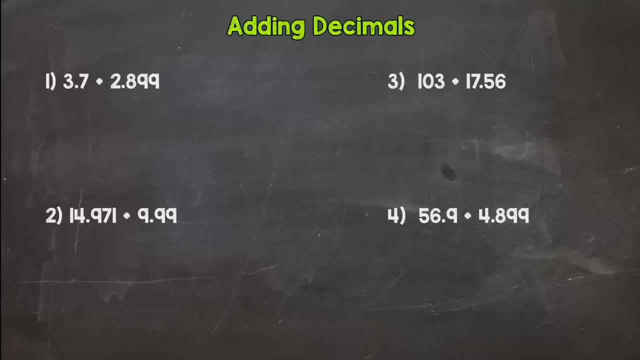 numbers. There's just one little rule, involved actually a couple little things, But if you have adding down and you're able to add, you'll be good with this. So the best way to learn about adding decimals is to go through some examples. 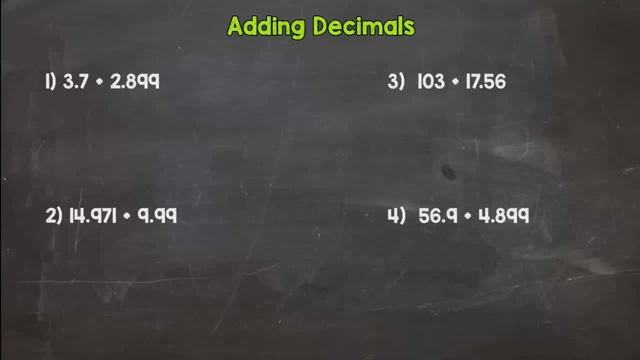 So you have two options. You can either write these problems out with me or just watch this video and then try some on your own afterwards. I would suggest writing these out with me. I think that will be more beneficial than just watching, but up to you. So let's start with number one And our first and 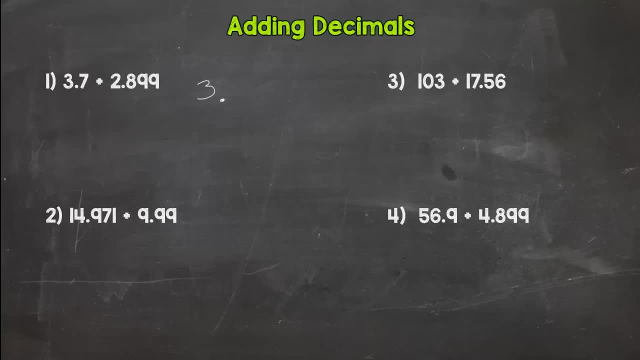 main rule is: when we add decimals, it's in the setup. here you need to line up your decimals And that will line up all of your place values for you, which is the important thing when it comes to adding decimals. So this is the 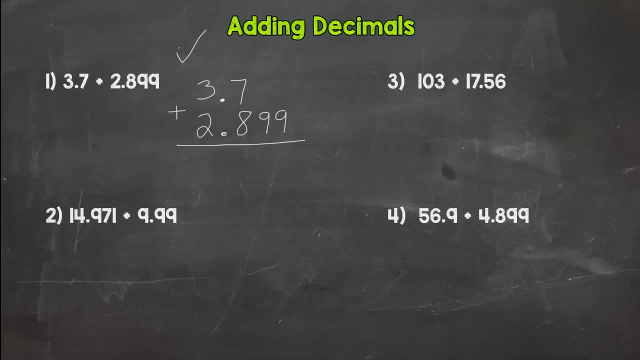 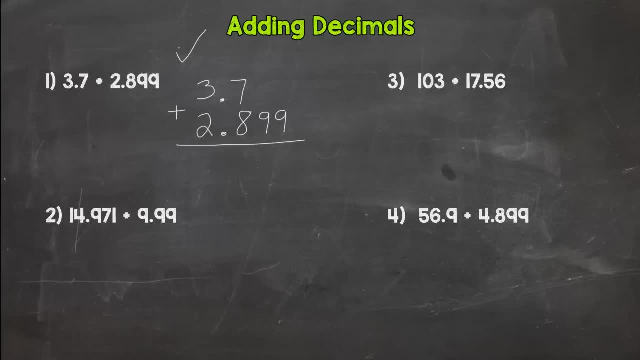 with the equivalent decimals. you know you can add zeros to the right of a decimal and it does not change the value. So I'm going to put a couple of placeholder zeros here. So both numbers go to the thousandths place And it's a little more lined up and looks a little better when it comes to. 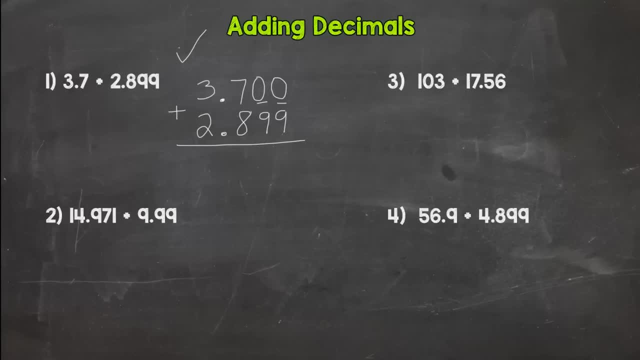 setting up this problem. Okay, so we would be good to go with adding. So now we just add 0 plus 9,, 9.. 0 plus 9, 9.. 7 plus 8 is 15.. 1 plus 3 is 4.. 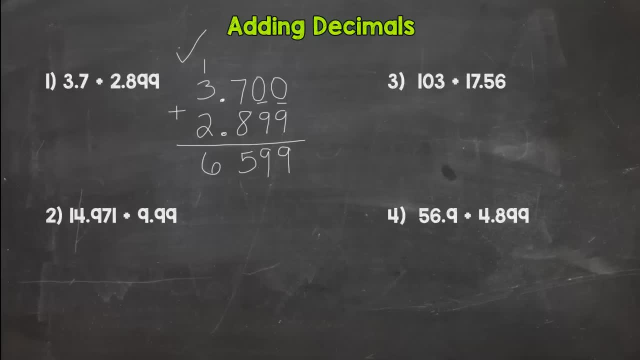 Plus 2 is 6.. Now we need to place the decimal in the answer. You can either do it as you go through the problem, which I'll do in number 2, or you can do it at the end. I personally like to do it as I go through the problem to make sure. 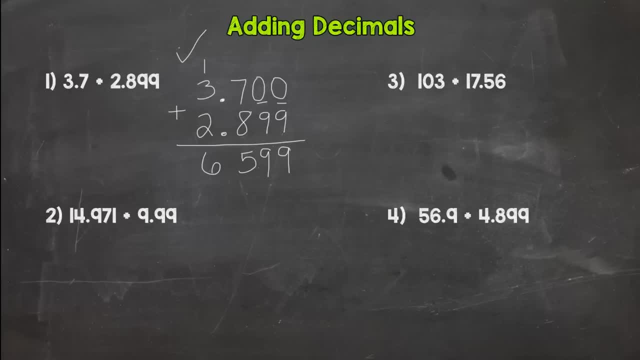 I don't forget it, But let's do it here. And you place the decimal by bringing it straight down with adding decimals, So it would go between the 6 and 5. And our final answer would be 6 and 599 thousandths, Now, always, whenever you're. 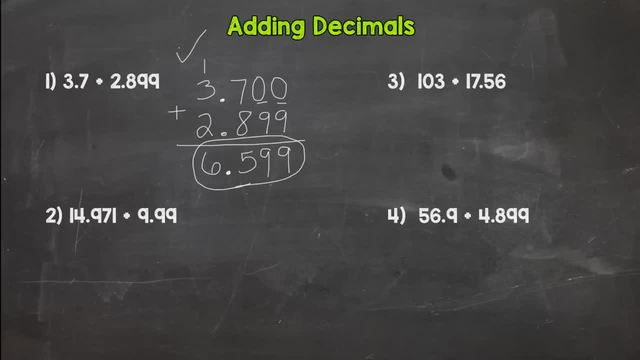 working with decimals or even whole numbers. check to make sure if your answer is reasonable or if it makes sense, And it only takes a couple of seconds. Use estimation and rounding. So 3 and 7 tenths is close to 4.. That's the. 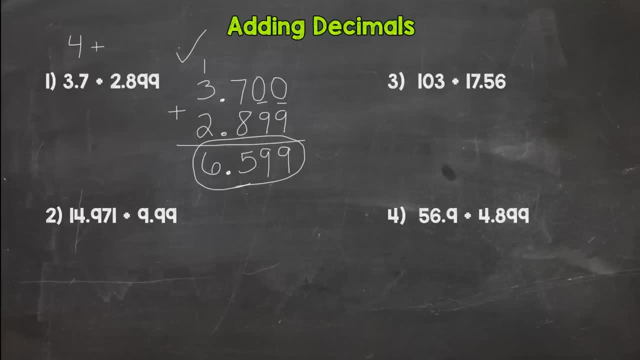 closest whole number. That's what it would round to, Plus 2 and 899 thousandths would round to 3.. So I'm just going to do a quick rounding and estimation: 4 plus 3 is 7.. So I know my answer should be close to 7.. If I'm not, something's off. 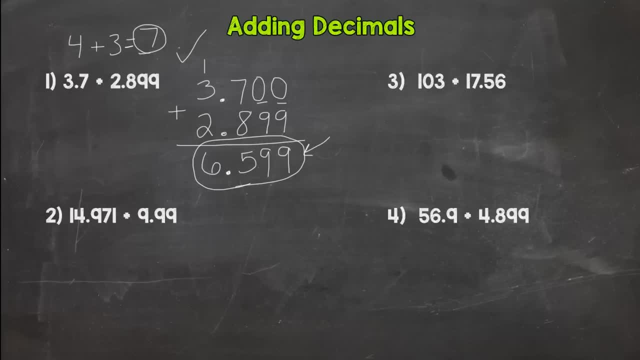 And my answer here is close to my estimation- Very close, So I have a reasonable answer. Okay, So line up your decimals, Use placeholder zeros, Bring your decimal straight down And just add. I'm going to show you one of the main mistakes over here to the left. This is not how you do. 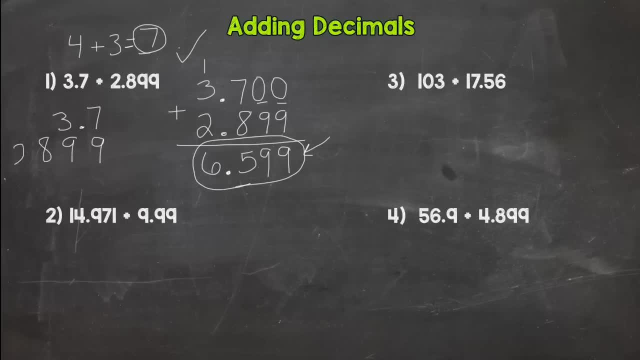 it. Add like this: lining just lining up your numbers. like that your places aren't lined up, your decimals aren't lined up. if you do that, you have no chance of getting the correct answer. okay, so let's go to number two. we're gonna speed it up a little bit here. line up your decimals. use placeholder zeros. if 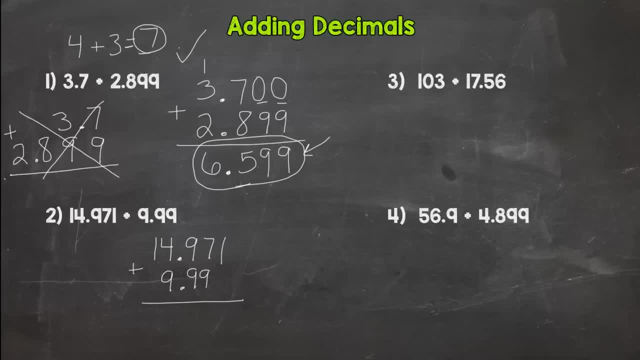 necessary. do you see where you can add a placeholder zero in right here? so they both go to the thousands. one, sixteen, nineteen, dot dot dot. bring that decibel straight down. one plus four is five plus nine is fourteen twenty four and nine hundred sixty one thousandths. let's do a little. 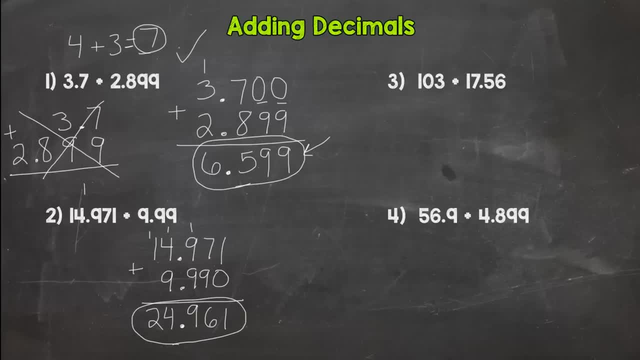 bit of estimation action up here. this would round the fifteen and that would round the ten, so our answer should be close to 25 according to our estimation, and our answer right here is very close to 25. so we have a reasonable answer and we lined everything up. so we are good to go. number. 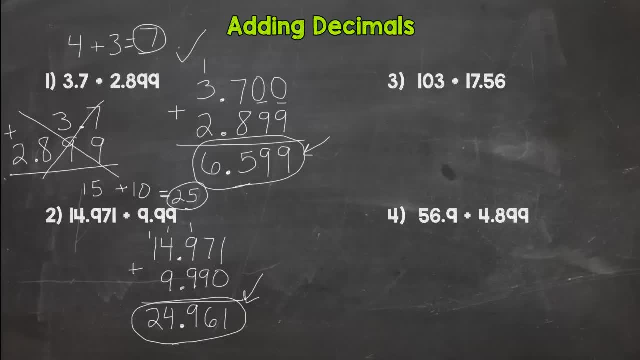 three is a very important problem because this is one of the main questions I get when it comes when we get to adding decimals. we have a 103 here and by now, hopefully you know we need to line up our decimals first. well, where does the decimal go for 103? because I don't see one. a decimal always comes. 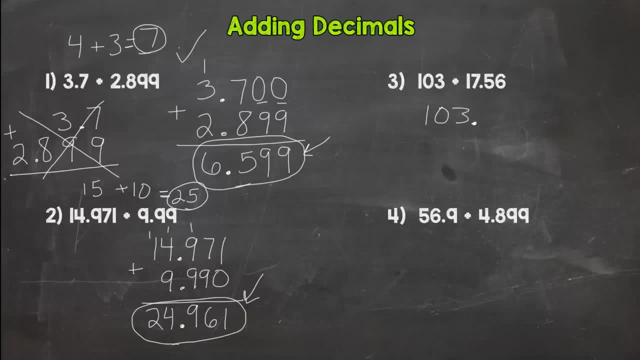 after a whole number. every single number has a decimal. never say 103 doesn't have a decimal. we just we just don't put it there because it's a whole number, we don't need it. but it can have one. put it afterwards. now we can line up 17 and 56 hundredths. it looks a little offset there, so I'm. 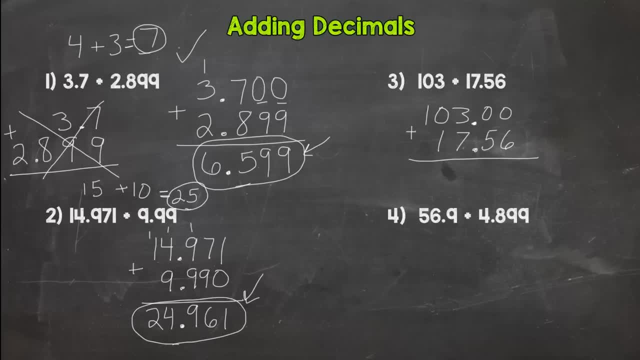 going to put in some placeholder zeros, and now I'm good to go with adding six, five dotdot hierarchies, P sidetrading on, and then one defteros, 120 and 56 hundredths- a little estimation up here. this is already a whole number, so I'll keep it at. 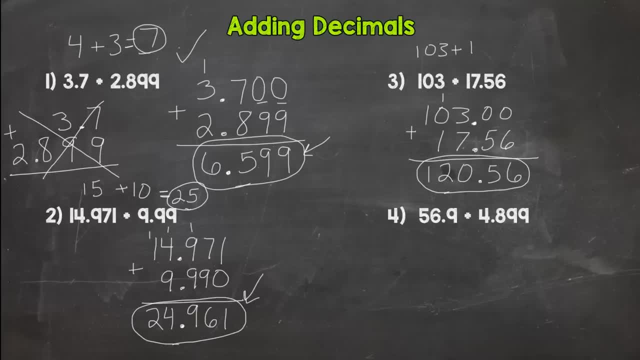 103, and then I'll run this to 18 and we get 121 is our estimation, and we are very close to that. so we have a reasonable answer. I'm gonna do a example over here of something that should set off a red flag if you accidentally- maybe you weren't neat with the setup or you accidentally put the decimal.